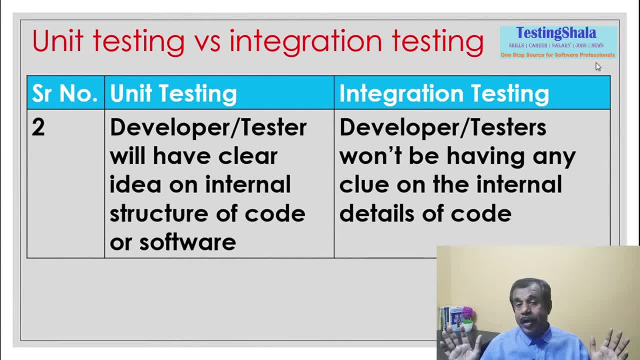 It has been done, They do not have any idea. The only thing is, once the integrations are done, I will be providing an input from this component. Then we will see, by passing all the component well, whether you will get an output in the third component or a second component, something like that. 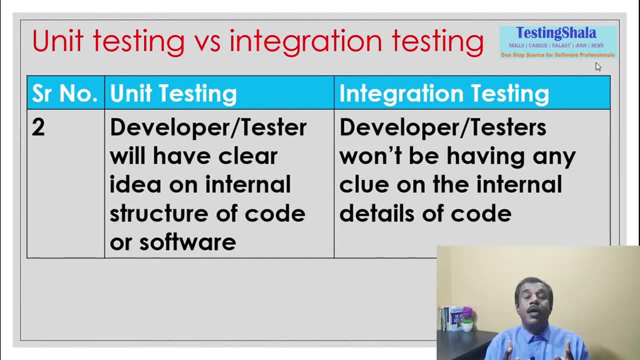 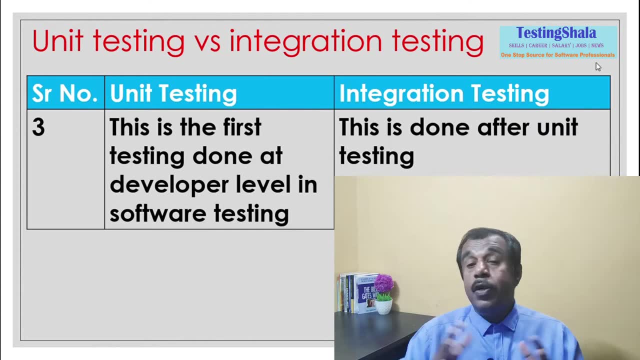 Here we do not have any idea on the component level, but the overall integration perspective. here we are doing in a block box perspective. In a block box perspective The integration testing will be done. The third difference is in the overall software testing Level software test. 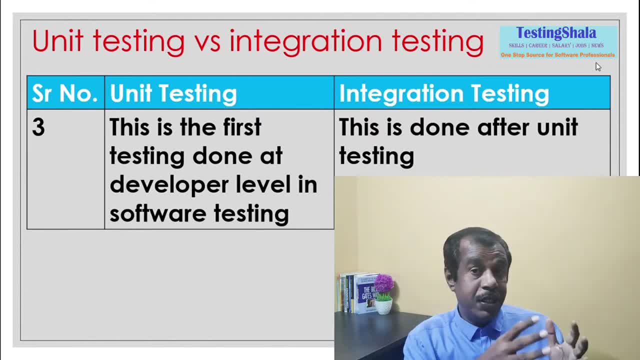 There are levels of testing is that? the first level of testing is a unit testing. The first type of testing we normally doing we do in a testing process is a unit testing. then, followed by the unit testing, We does the integration testing, which is the second type of testing, which we call as a unit testing. 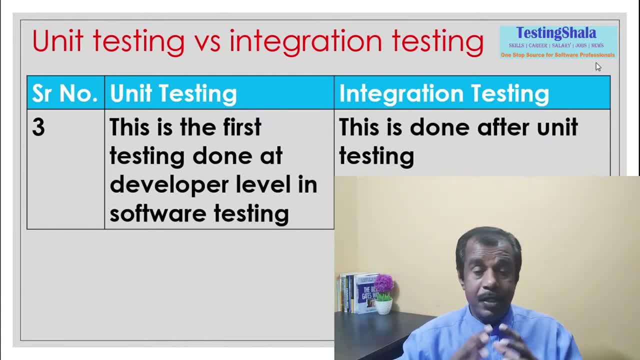 The third type of testing, which we call as a integration testing. that is a major difference between unit and integration, As I said earlier. the fourth major difference is unit testing is completely. We also call it as a glass box testing or a gray box testing. 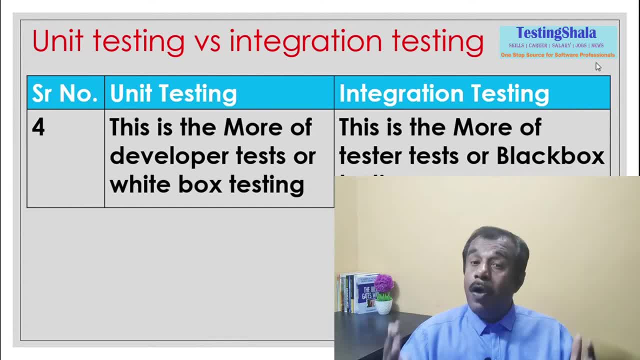 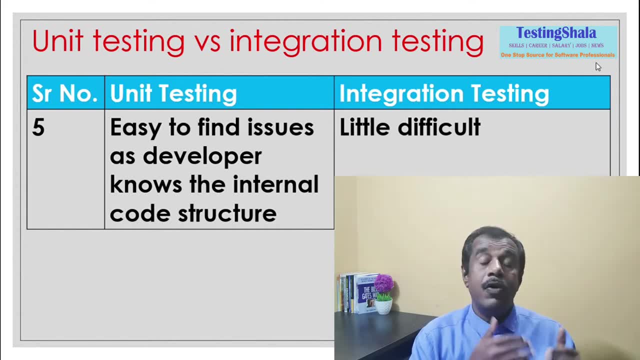 But integration testing, we call it as a block box testing. The fifth major, fifth major difference is in the unit testing. for the developer, Because he knows how the code has been written and based on that he has written the test cases. For him things are little simpler because by watching the code he will be writing the test cases. 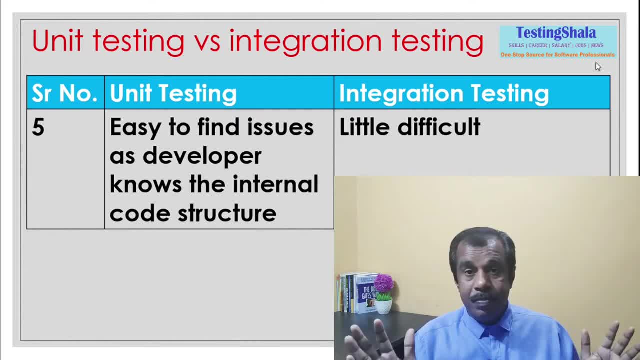 But for integration test cases it is not something like that. The things will become very complex because if they are involved, lot of dependencies, lot of integration points, lot of flow of information from one network, lot of flow of information from one network. 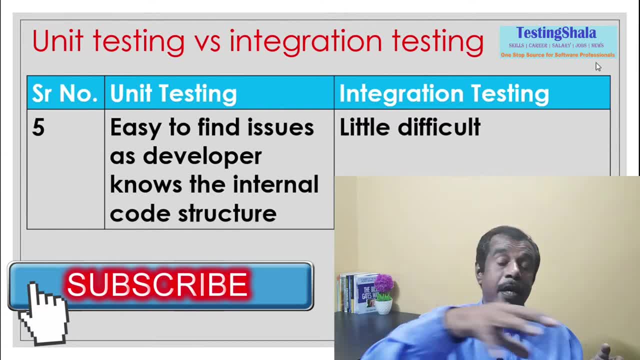 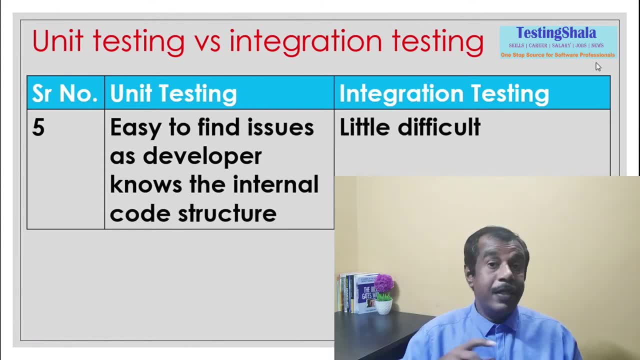 lot of flow of information from one network, One model, to another model, how the different data types are moving, how the data is moving from one place to another places. As the complexity increases, the integration testing becomes little higher complexity compared to unit testing. 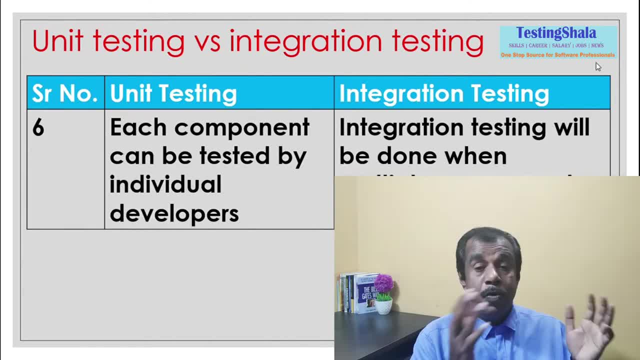 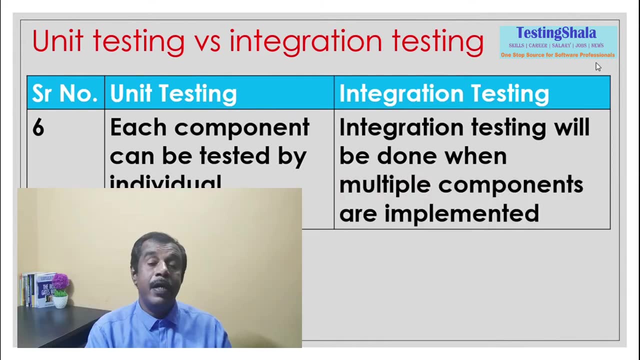 The sixth main important difference is: sixth main important difference is: small component has been implemented. When the small component has been implemented, then the unit tests are developed. Integration: if multiple modules or multiple components are implemented, then only we will be bringing integration testing to be tested there. 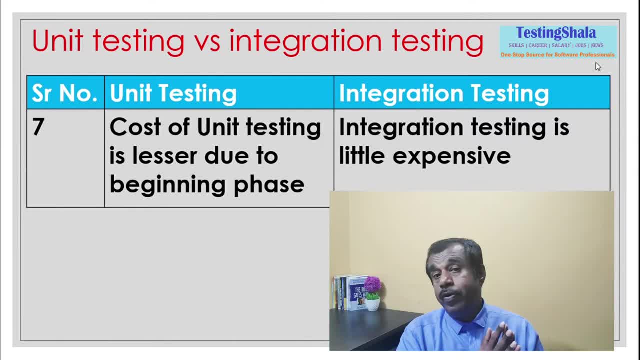 The seventh important difference is the cost of doing a unit. testing is little cheaper because it happens in the beginning And if any issues find out during that phase is easy to fix and the cost is also little lesser when you are doing everything in the beginning. And if any issues find out during that phase, is easy to fix and the cost is also little lesser when you are doing everything in the beginning As we move on to the next phase. if some issues are popped up, and any issue which will come in this area, then anything it requires fixes. it requires lot of money as well. As we move on to the next phase. if some issues are popped up and any issue which will come in this area, then anything. it requires fixes. it requires lot of money as well As we move on to the next phase. if some issues are popped up and any issue which will come in this area, then anything it requires fixes. it requires lot of money as well. As we move on to the next phase. if some issues are popped up and any issue which will come in this area, then anything. it requires fixes. it requires lot of money as well As we move on to the next phase. if some issues are popped up and any issue which will come in this area, then anything it requires fixes. it requires lot of money as well. 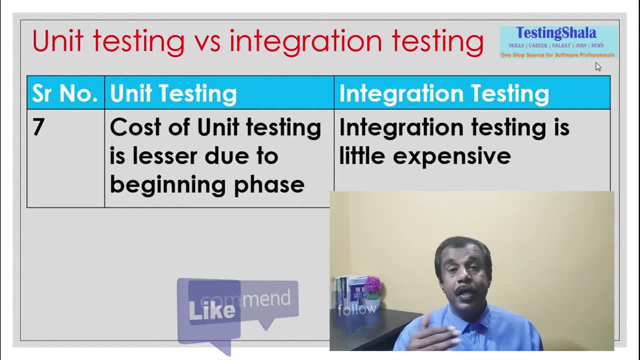 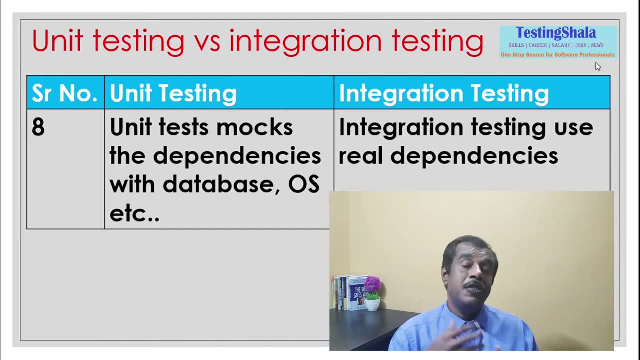 As we move on to the next phase. if some issues are popped up, and any issue which will come in this area, then anything it requires fixes. it requires lot of money as well. Integration Testing is little expensive compared to Unit Testing. Eighth difference is: in the Unit Testing normally we write stops or programs or subroutines to create a dependencies or create an output file or create an input file. 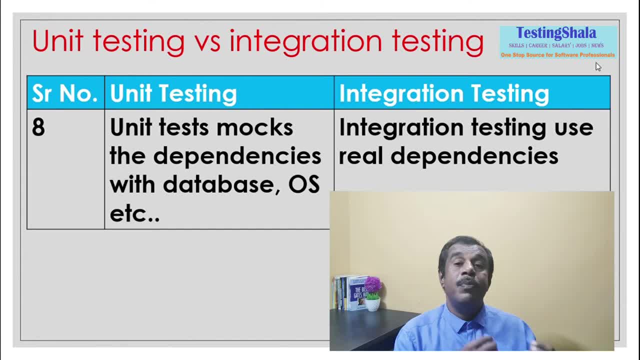 Eighth difference is in the Unit Testing. normally we write stops or programs or subroutines to create a dependencies or create an output file or create an input file. Then from there we pick the information, where we normally mock up the databases, we mock up the input files, we mock up. 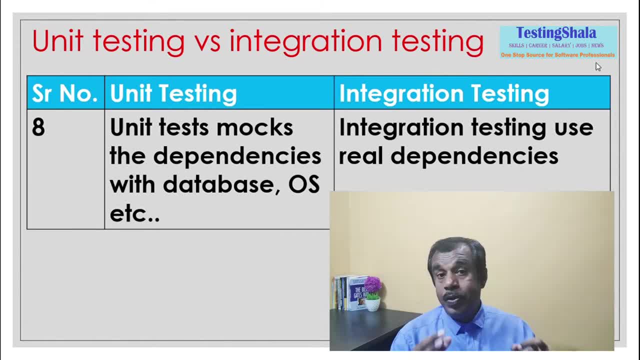 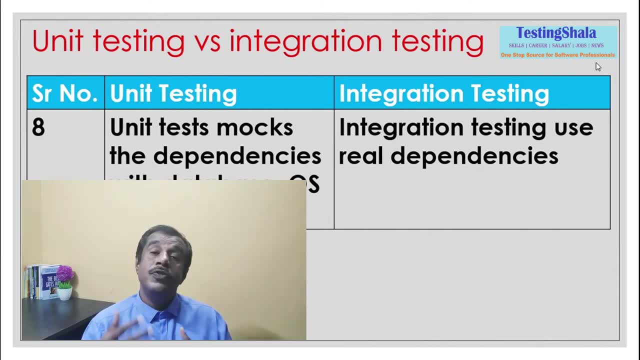 the various aspects when we are testing unit test cases. but in the integration testing we are really trying to test practically where which module is been integrated to other module. is there any third-party modules are there? whether this model is integrated with the third-party applications, every aspects. 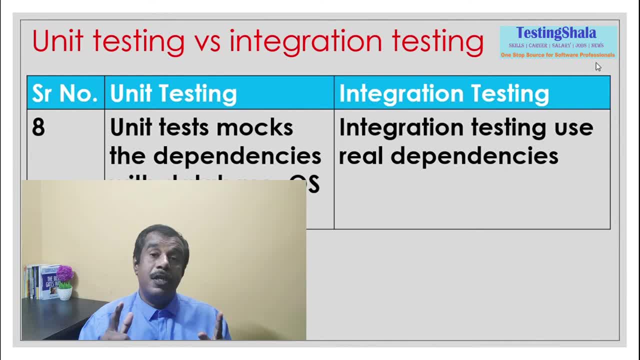 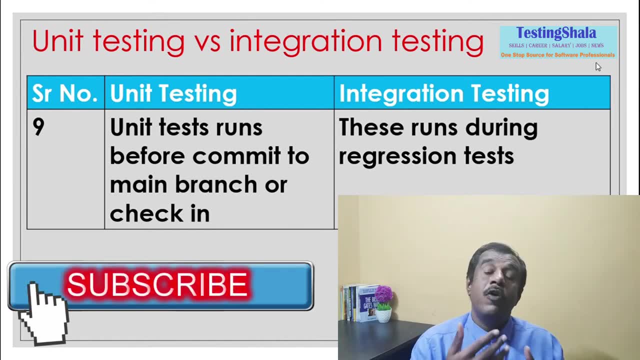 will be testing as part of the integration testing, unit test cases. normally we ran unit test cases. we normally ran. whenever developers completes a particular components, he goes and checks in the code into the system- it could be GitHub or anywhere. if he is trying to check in, that is the. 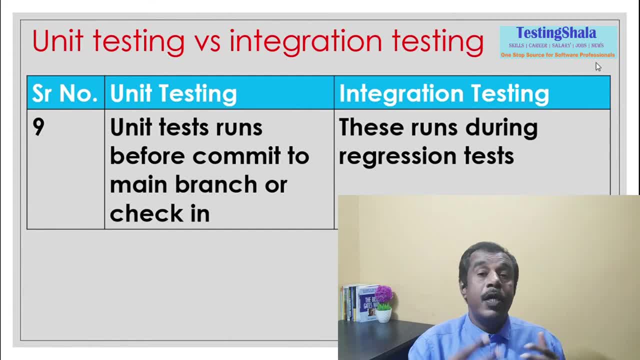 time this unit test will run just to ensure that whatever the new component has been implemented is not broken. that is where the unit testing will come into picture. but integration test cases: as and when the multiple modules are getting integrated. multiple components are getting integrated into the code base. that is the time the integration 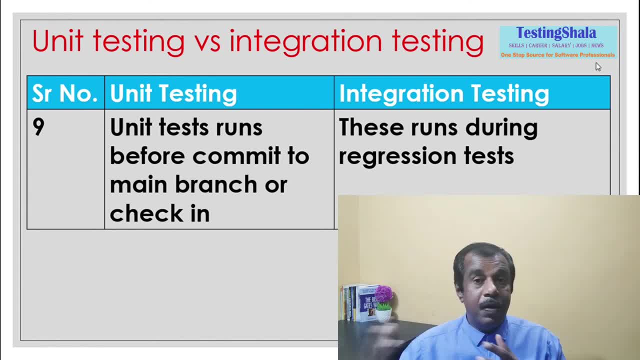 regression test cases will be keep running as and when more components are getting integrated each other. so we will be writing more test cases and also will be executing more integration test cases, just to ensure that all the integration points between one component to another component that really works there. the 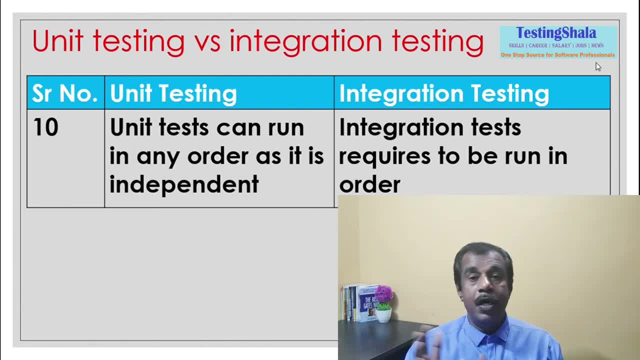 tenth important major difference between unit testing and major difference between unit testing areas. unit testing: all the test cases are independent enough. they are totally independent. there is no dependency because individual component: if I want to test, if I execute those tests, my job is done. but in the integration, because we have to test in a particular order, randomly. 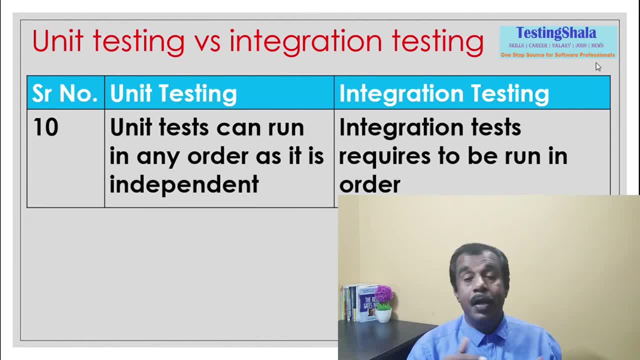 contested in unit testing any test cases separately. but if I wanted to execute the tests in integration level, then we should come with the order, because there is a dependencies will be there. there is a flow of data between one model to another model is there? lot of integration aspects will be there. hence we'll have to execute the test cases in a particular order. that is a major difference between unit test cases and integration test cases. at least I am hoping. now I have given ten important difference between unit and integration testing. I am hoping you guys really got to know a lot of information. 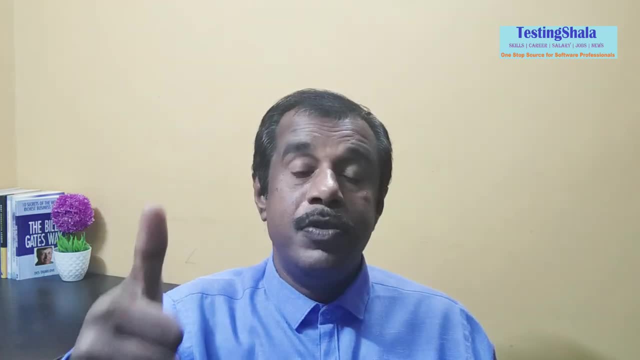 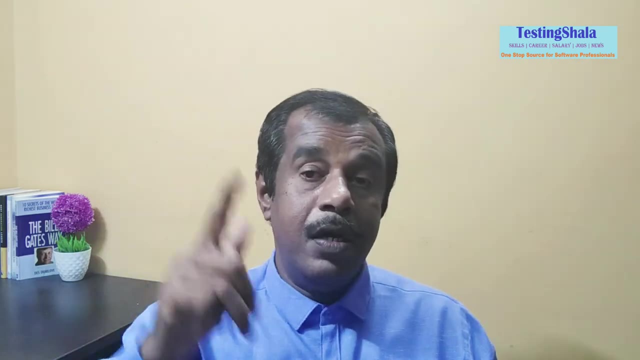 from this video. if you really like this video, then please give a thumbs up to this video. if you guys are not subscribed to testingshala youtube channel, then please click on subscribe and bell icon so that all our future videos will be in your inbox. thanks for watching this video. bye for now. take care.